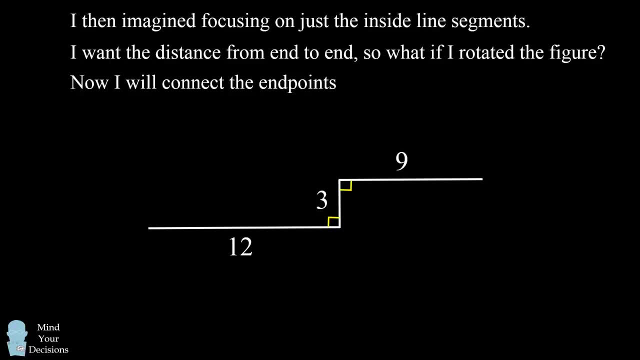 Then it struck me, I connected the endpoints of these line segments and then I realized we basically have one large right triangle. I can move the length of 9 down to form one leg of this right triangle, and then I can move the length of 3 over to create another leg of this right triangle. 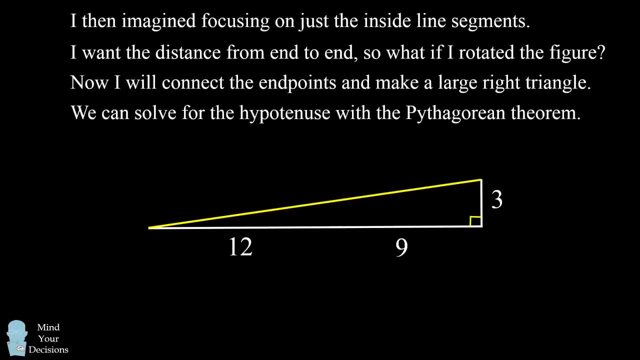 So we can then solve for the distance using the Pythagorean theorem. We have one leg of the triangle, that's 12 plus 9, or 21,, and another leg which is 3.. So the length of the hypotenuse is the square root of 21 squared plus 3 squared. 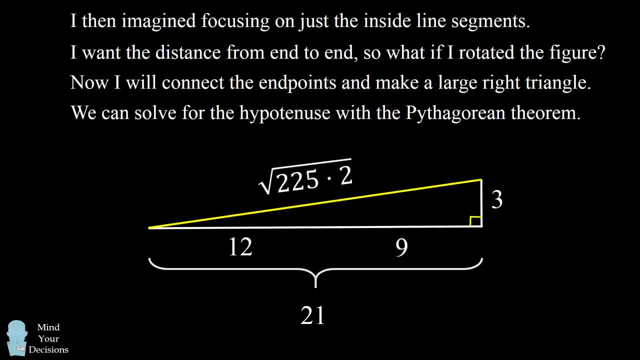 This becomes the square root of 450,, which is also equal to the square root of 225 times 2,, which then becomes 15 times the square root of 2.. So now let's take this information and get back to the original diagram. 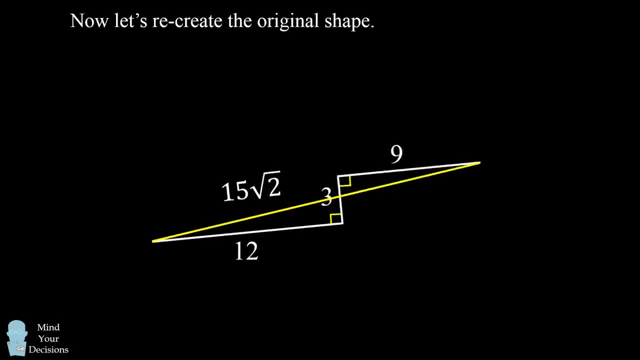 We'll recreate our line segments on the interior of the square and then we'll rotate them so that we have the distance from one corner of the square to the other corner of the square. We know the diagonal of the square is 15, square root of 2,. 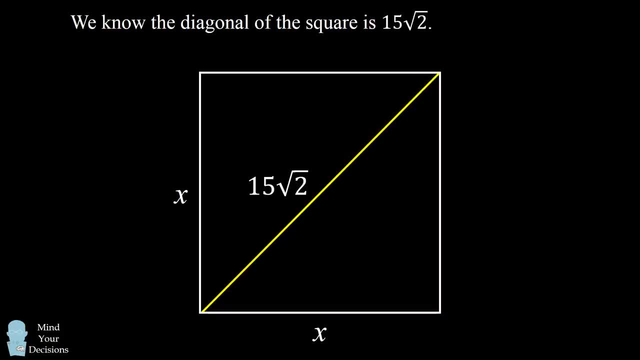 that's 15 squared over 2.. That's what we calculated, And now we also know that the diagonal of the square is x times the square root of 2.. This is because the diagonal of the square is the hypotenuse of a right triangle. 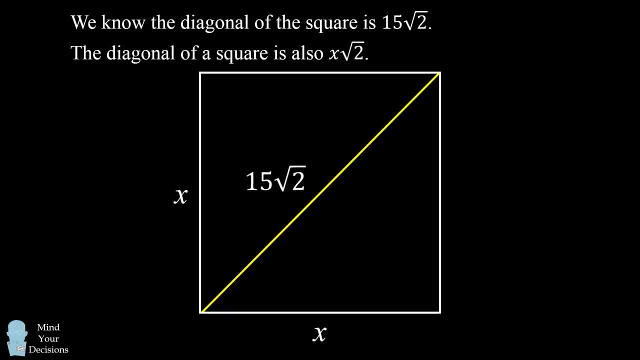 with two legs that are each x, So we can set 15 square root of 2 to be x times the square root of 2, and we can solve that x is equal to 15.. And that's our answer. So it took a little bit of work, but it was a lot of fun. 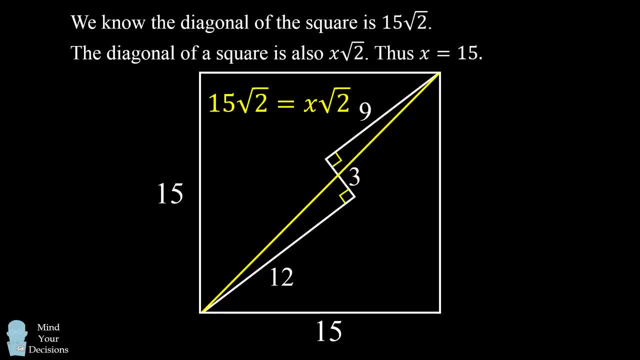 It took a lot of work to figure out what the length of this square side is, And sometimes in these problems you have to approach them in more than one attempt. In this problem, it took me three attempts before I could solve it. Did you figure out this problem? 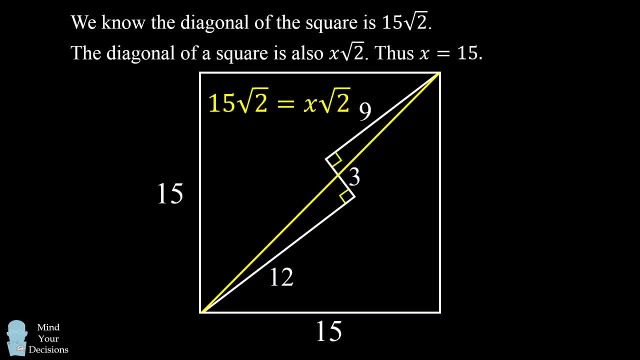 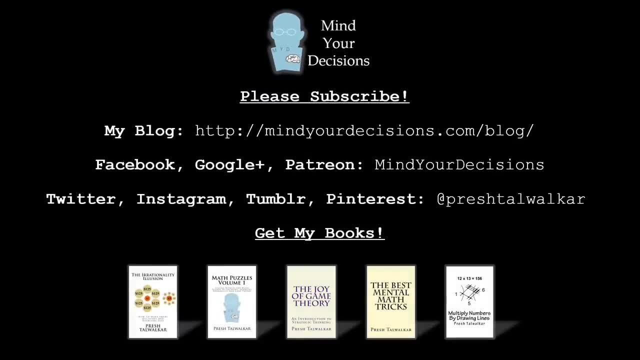 And did you come up with another solution? Thanks for watching this video. Please subscribe to my channel. I make videos on math and game theory. You can catch me on my blog Mind Your Decisions, which you can follow on Facebook, Google Plus and Patreon. 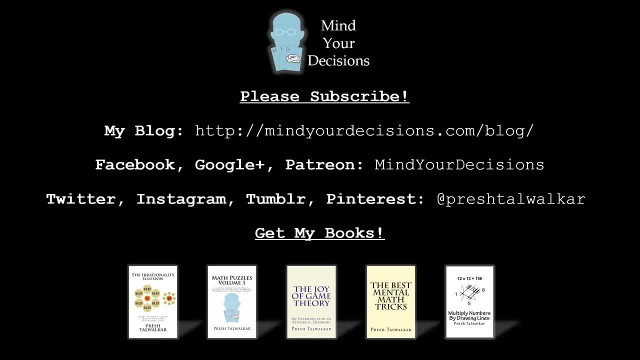 You can catch me on social media apps and social media And, if you like this video, please check out my books. There are links in the video description.